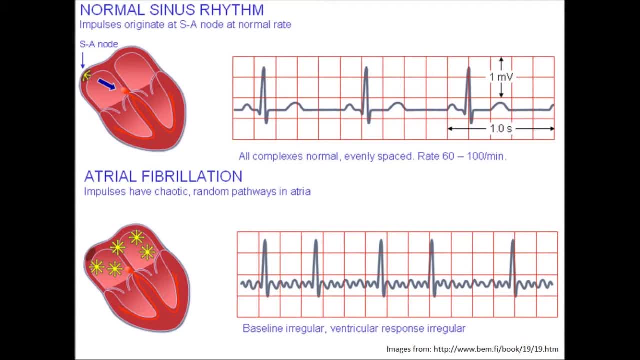 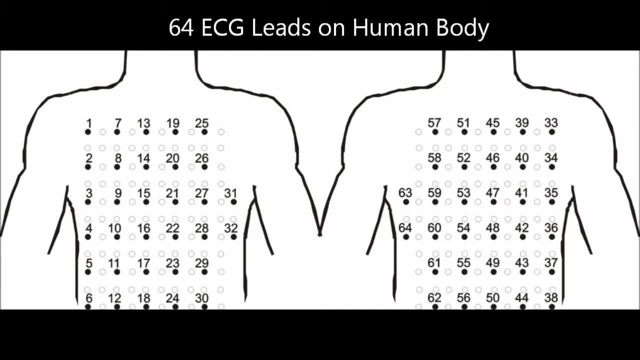 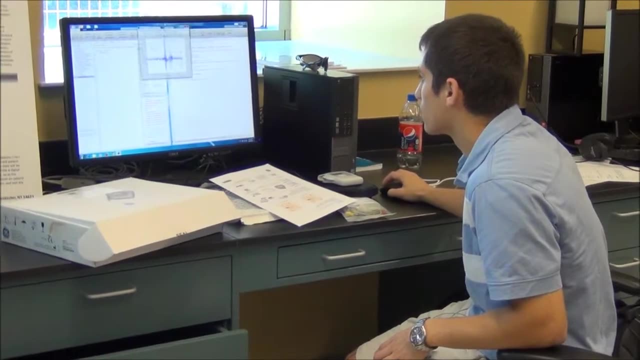 also a few other smaller waves before the QRS complex occurs. So we're just trying to see where we can put these leads and easily detect that a patient has atrial fibrillation. I usually just, you know, come into the lab, sit on the computer, open up MATLAB, start. 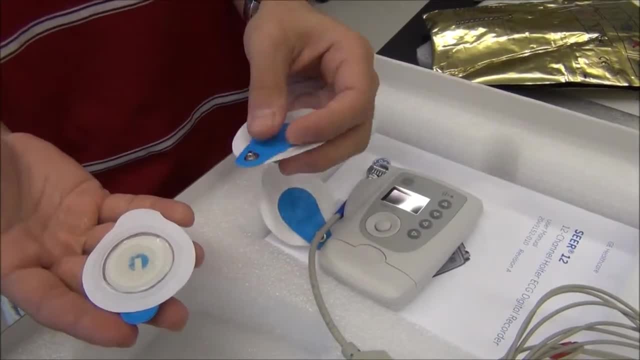 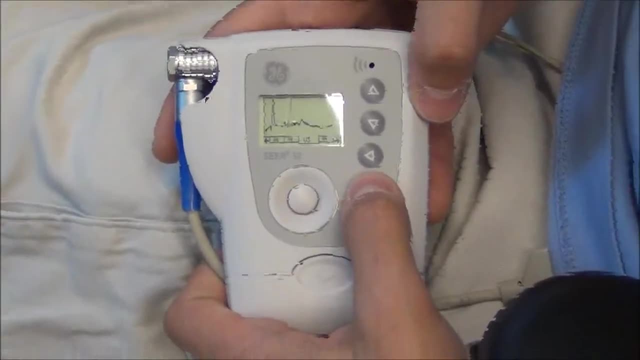 looking at the signals: Currently, when we have that GE Holter recording device, I began working with that so that was a little bit more hands-on, but mostly it's just analyzing signals in MATLAB. GE has that diagram on there and these precordial. 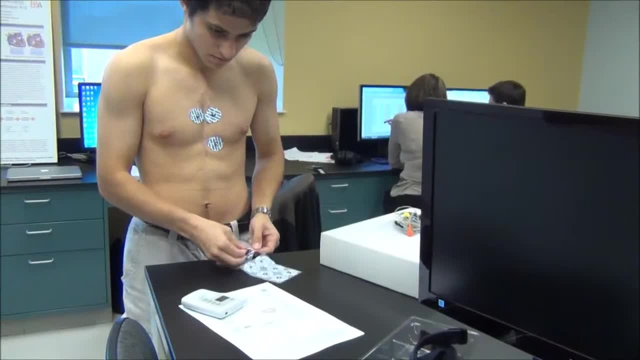 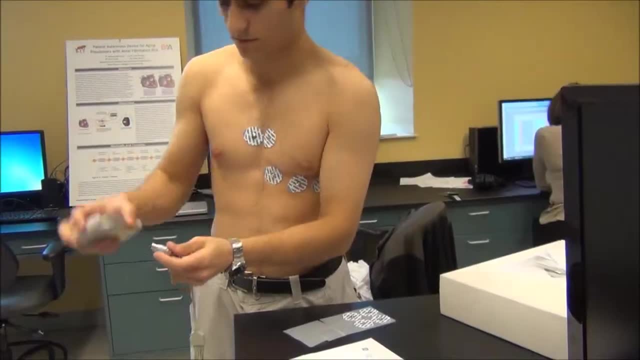 leads are standard V1 through V6, as was shown, with me hooking that up. The other four they go: two on the collarbone and two on the bottom of the rib. The reason those are there is because the device that we purchased from GE, that is. 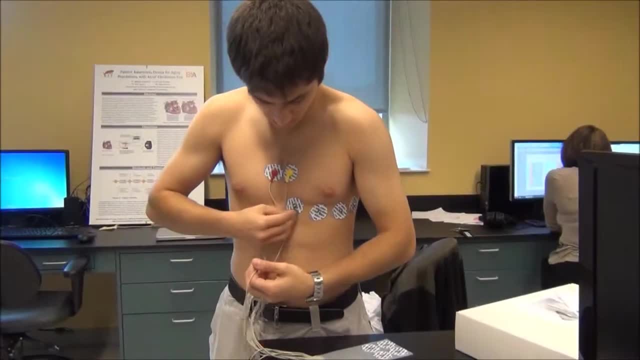 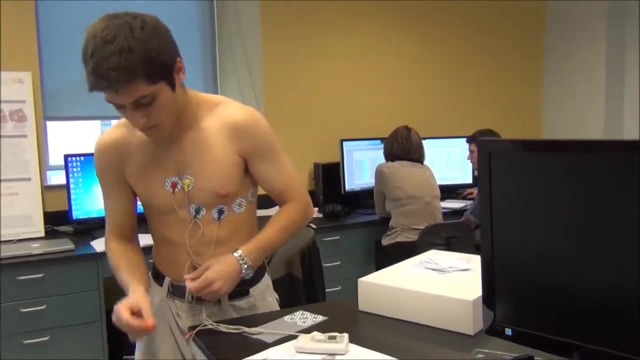 a portable device and for a patient to have that on for a day or two days in a row would be problematic if you actually had the leads on the wrists as well as the arms. We have data from a hospital in the UK. We only have 20 patients so far, so it's 10. atrial fibrillation. 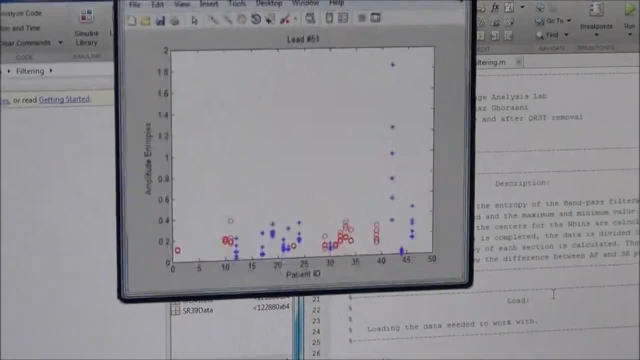 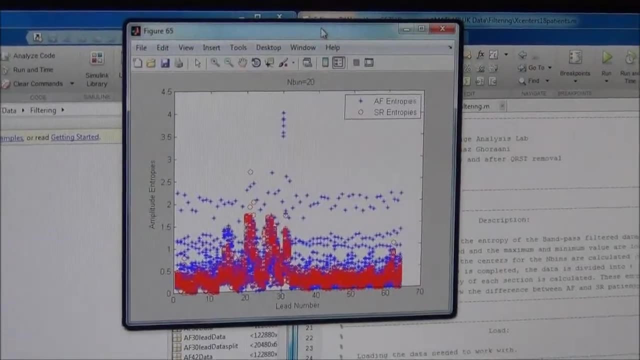 and 10 sinus rhythm patients. We have one-minute ECG recordings of each of the leads, maybe on that 64-lead dial. We have a lot of data on that, but we don't have a lot of data. We have a diagram. What we're doing is running that through a filter that we generated in. 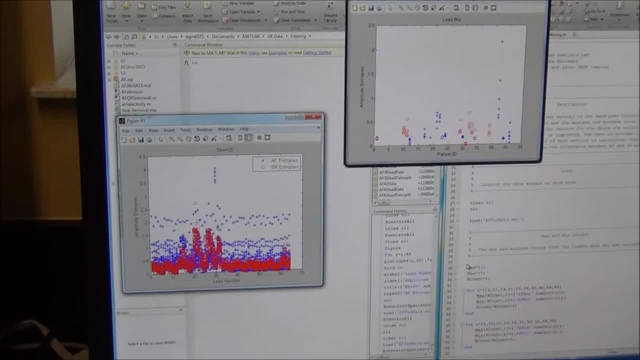 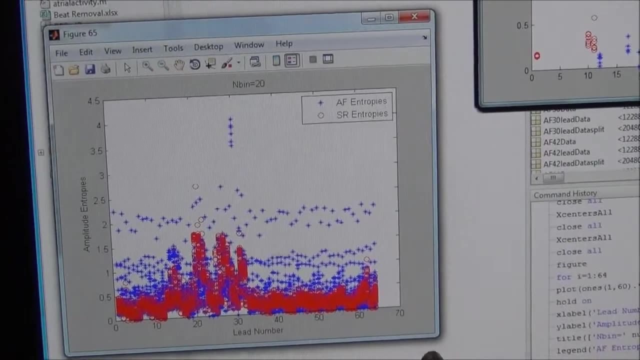 MATLAB and the filter we generate is based on papers we've read that remove baseline wander as well as reduce the noise of the signal. And after we've run it through a filter we start analyzing it and we're specifically doing entropy analysis on them to see if patients 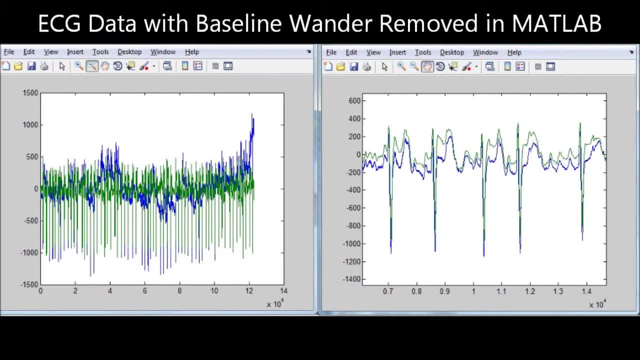 who have atrial fibrillation have a higher entropy than patients who have normal heart beating. When I was born I had some heart problems. So when I was two, I had a heart attack. I had a heart attack. I had a heart attack. 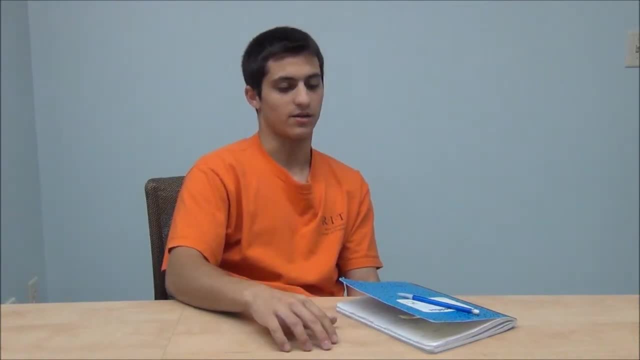 two years old I had my first open heart surgery And then, at nine years old, I had another heart surgery. So ever since growing up and being in and out of the hospital, I've just gotten used to and I've been very interested in the technology behind biomedical instrumentation.